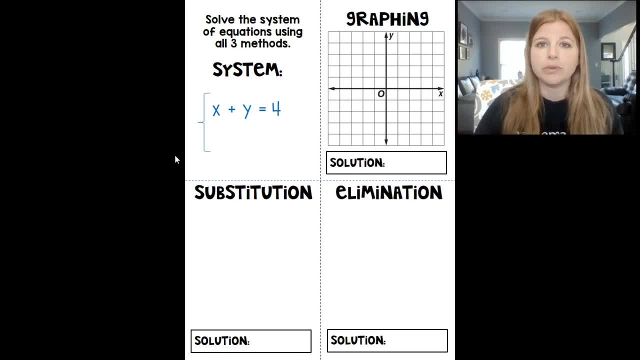 of x plus y equals 4, a nice equation. that's in standard form. and this other equation, y equals 2x minus 2, which is in slope-intercept form. we're going to solve this system, we're going to get our solutions and again, we're going to see something very special about the solution. 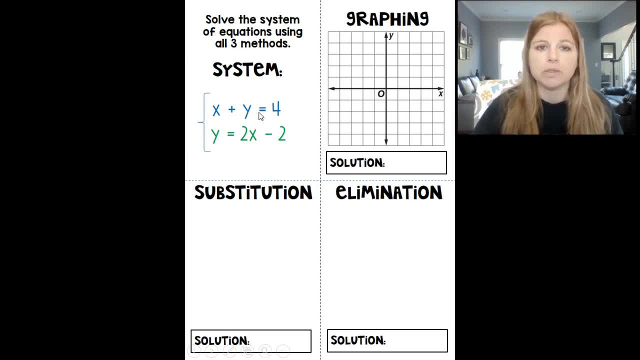 So first I'm going to graph this equation of x plus y equals 4.. Now there's a couple things I could do for graphing. I could either rearrange this equation and put it into slope-intercept form and then graph it that way, or, when it's in standard form, it's actually really nice to find. 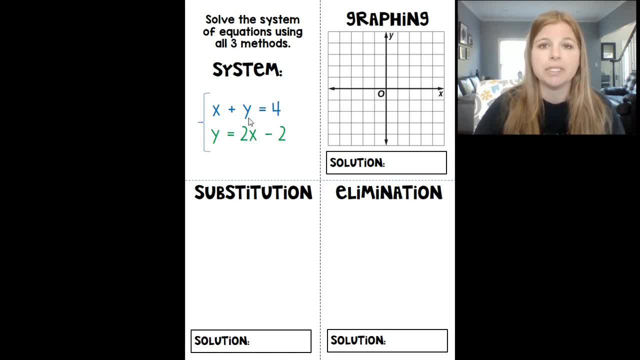 the intercepts. Remember to find the x and y intercept. you simply plug in a 0 for x and then a 0 for y. So if I was to go ahead and plug in a 0 for x, 0 plus y equals 4.. So if I plug in a 0, 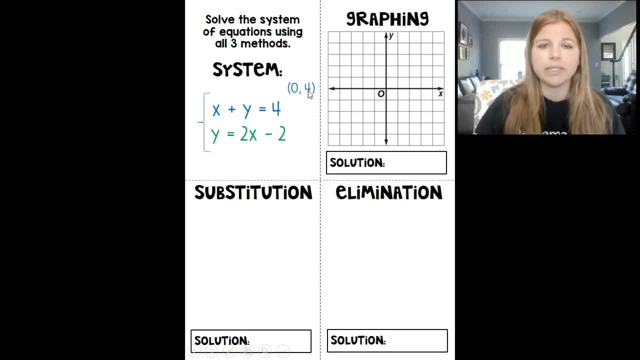 for x. that means the y has to be 4.. 0, 4 is one of my intercepts, and it would be right here If I plug in a 0 for y. x plus 0 equals 4.. That would mean that x is actually 4.. So my intercepts: 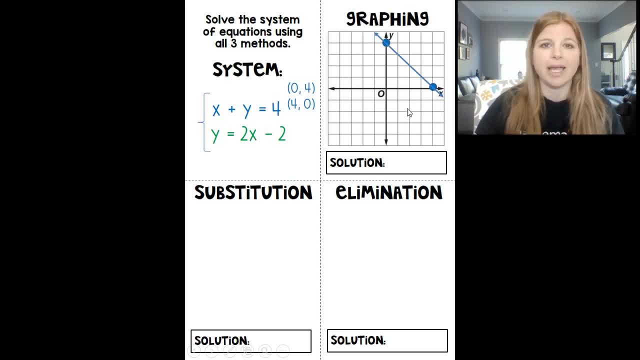 are 0,, 4, and 4, 0. And if I connect those points I get that nice line. If I had rearranged this equation it would have looked like y equals negative x plus 4.. So y intercept at 4, a slope. 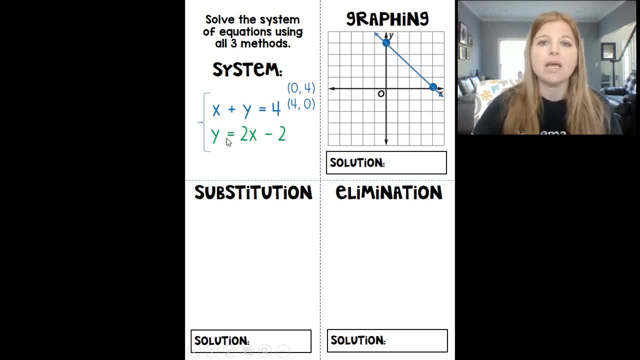 of negative 1, and I would get the exact same line. The next one is in slope-intercept form. so let's graph that. We know we plot our y-intercept first at negative 2.. We then plot our slope of 2,, so up 2 to the right 1, up 2 to the right 1, up 2 to the right 1.. And then from: 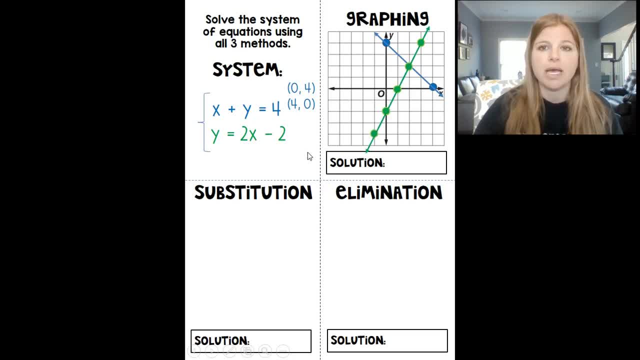 that y-intercept. I'm going to go ahead and go down 2 to the left 1, and then draw my line. I can see pretty clearly where the intersection is. That's the key for a graph is seeing where the two lines intersect each other. It's at this coordinate point. 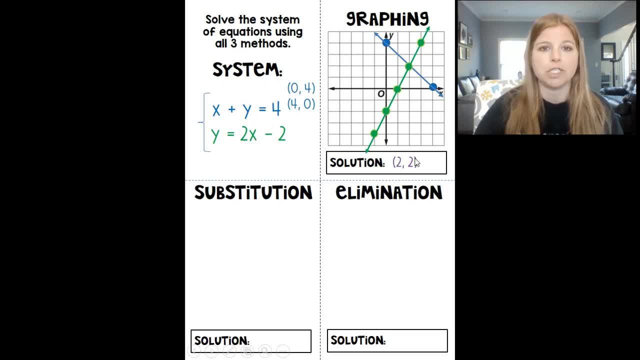 The coordinates are 2, 2, and that's my solution. If I went ahead and plugged 2, 2 into the equation, 2 plus 2 is 4. It works. If I plug in 2 here, 2 is equal to 2 times 2.. It's a lot of 2s here. 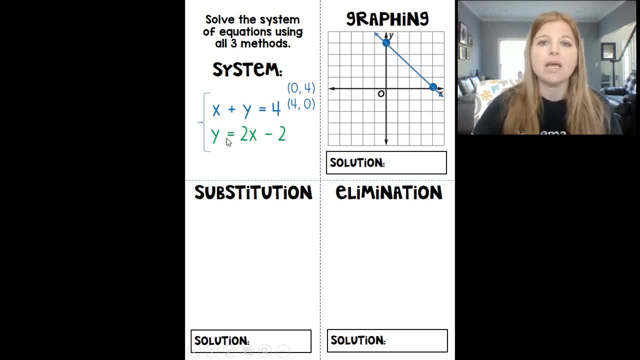 of negative 1, and I would get the exact same line. The next one is in slope-intercept form. so let's graph that. We know we plot our y-intercept first at negative 2.. We then plot our slope of 2,, so up 2 to the right 1, up 2 to the right 1, up 2 to the right 1.. And then from: 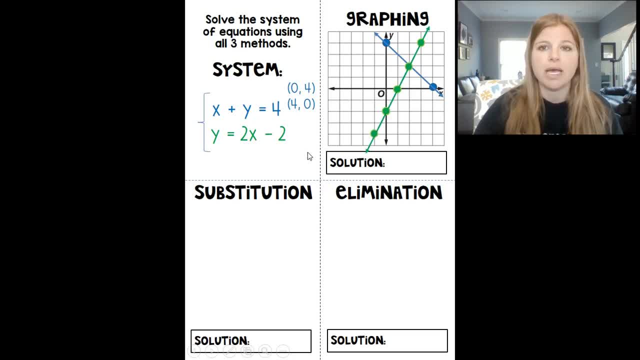 that y-intercept. I'm going to go ahead and go down 2 to the left 1, and then draw my line. I can see pretty clearly where the intersection is. That's the key for a graph is seeing where the two lines intersect each other. It's at this coordinate point. 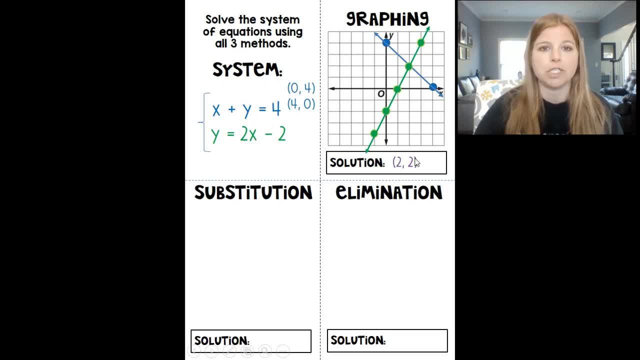 The coordinates are 2, 2, and that's my solution. If I went ahead and plugged 2, 2 into the equation, 2 plus 2 is 4. It works. If I plug in 2 here, 2 is equal to 2 times 2.. It's a lot of 2s here. 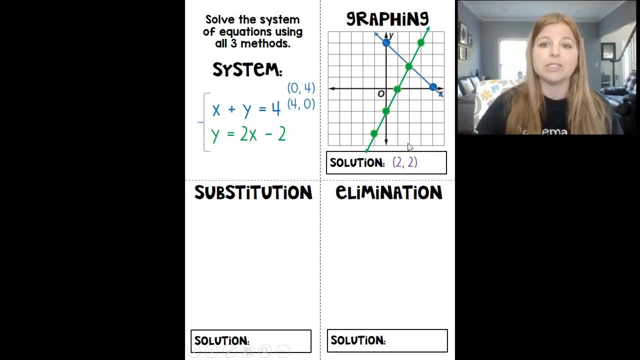 2 times 2 is 4.. 4 minus 2 is that 2.. So if I plug this solution, this 2, 2, back into my original equations and I get true statements, I know it's good Now. substitution, Substitution. 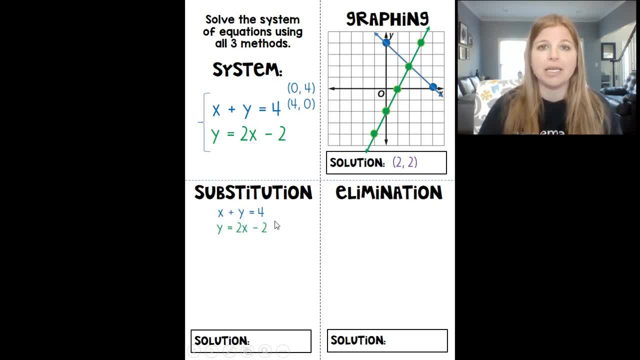 is a method Where we want one of the equations to be set equal to a variable. This first equation- x plus y equals 4, is not set equal to a variable. I don't have x or y by itself, But look at: 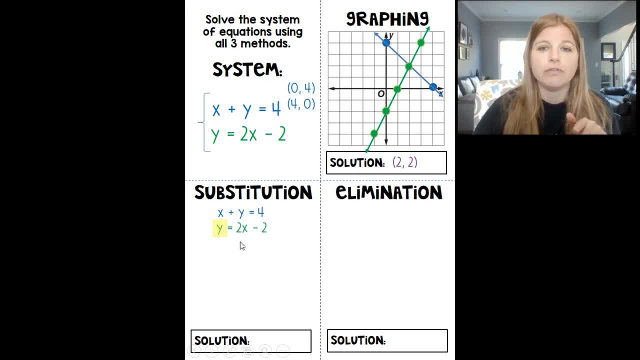 the second equation. This is actually already set up for y to be by itself. y is equal to 2x minus 2, and I have it highlighted there for us. So that means, wherever I see y in my other equation, I'm going to substitute in everything that y is equal to in for that. 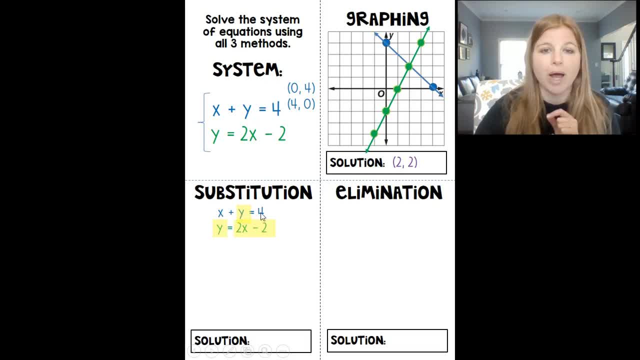 y. So instead of this equation looking like x plus y equals 4,, it's going to say x plus 2x minus 2 equals 4.. Now I want you to really see what's happening here. y is equal to the. 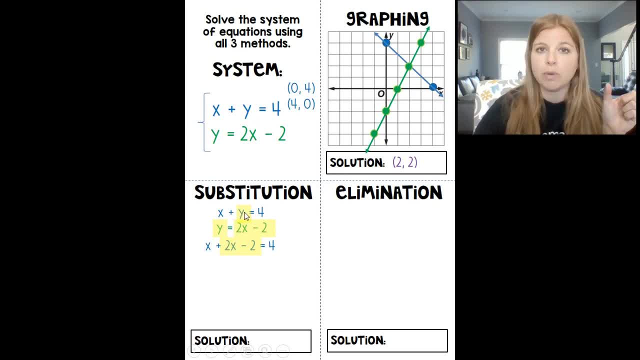 entire expression of 2x minus 2.. So wherever I see y in my other equation, I'm going to substitute that. all in So if you look at this first line and you look at this new line here, from the first line to the third line, you can see the y was replaced or substituted with that. 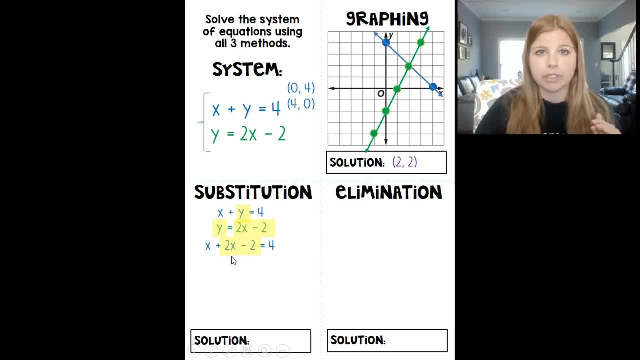 2x minus 2.. And now I've got just a basic multi-step equation to solve guys that we've been solving for years. So x plus 2x is 3x. I'm going to go ahead: add 2 on both sides. 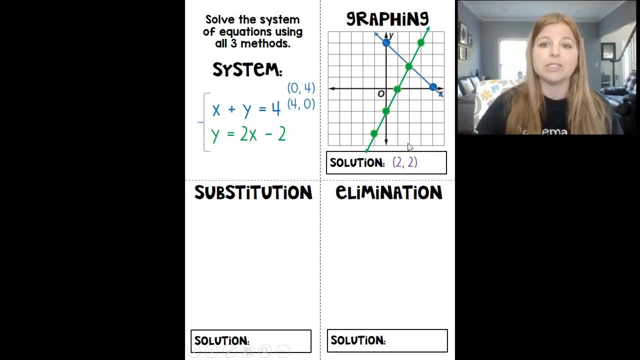 2 times 2 is 4.. 4 minus 2 is that 2.. So if I plug this solution, this 2, 2, back into my original equations and I get true statements, I know it's good Now. substitution, Substitution. 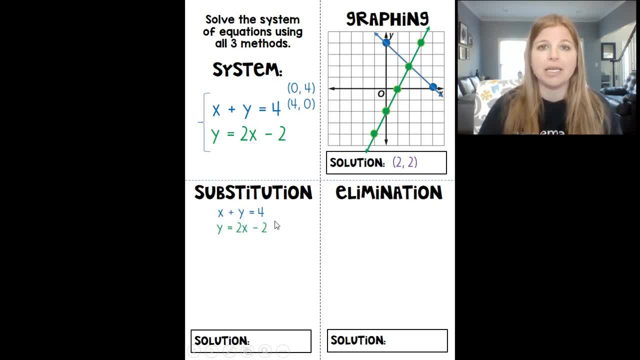 is a method Where we want one of the equations to be set equal to a variable. This first equation- x plus y equals 4, is not set equal to a variable. I don't have x or y by itself, But look at: 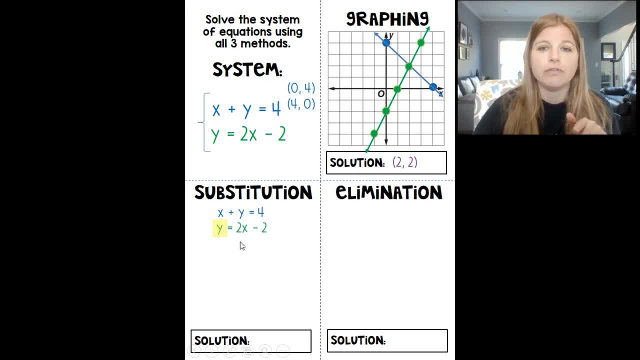 the second equation. This is actually already set up for y to be by itself. y is equal to 2x minus 2, and I have it highlighted there for us. So that means, wherever I see y in my other equation, I'm going to substitute in everything that y is equal to in for that. 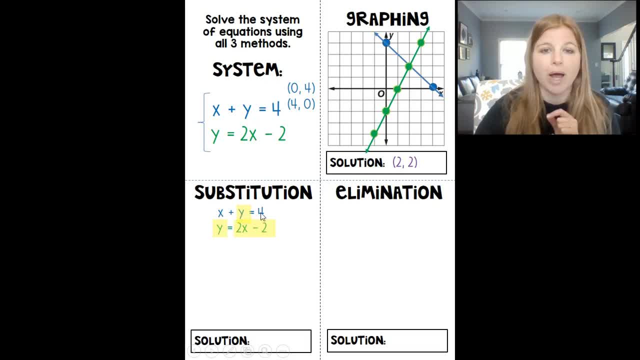 y. So instead of this equation looking like x plus y equals 4,, it's going to say x plus 2x minus 2 equals 4.. Now I want you to really see what's happening here. y is equal to the. 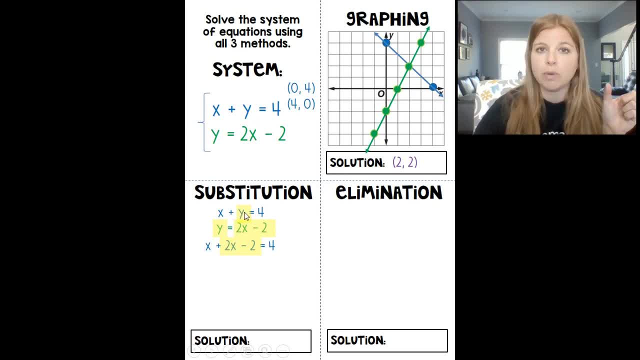 entire expression of 2x minus 2.. So wherever I see y in my other equation, I'm going to substitute that. all in So if you look at this first line and you look at this new line here, from the first line to the third line, you can see the y was replaced or substituted with that. 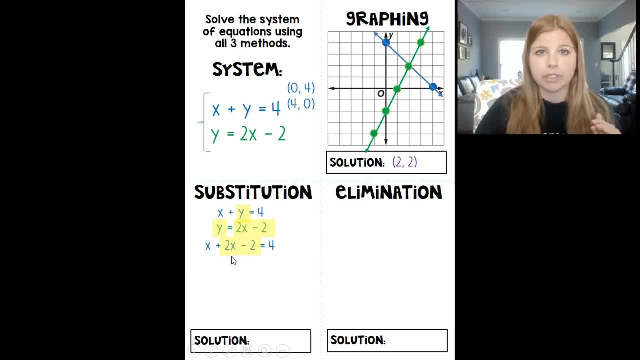 2x minus 2.. And now I've got just a basic multi-step equation to solve guys that we've been solving for years. So x plus 2x is 3x. I'm going to go ahead: add 2 on both sides. 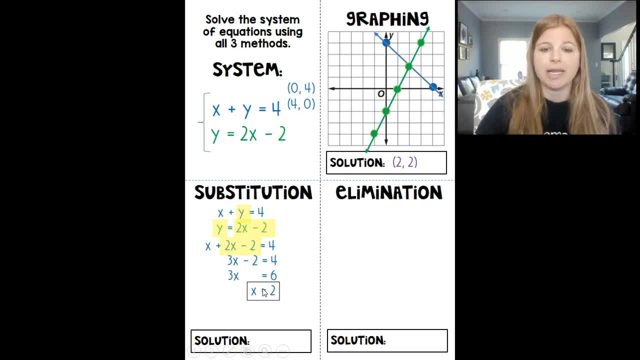 to get 3x equals 6,, divide both sides by 3, and x equals 2.. And that's wonderful. But let's remember the solution. when we graphed it was an ordered pair: It's an x and a y. 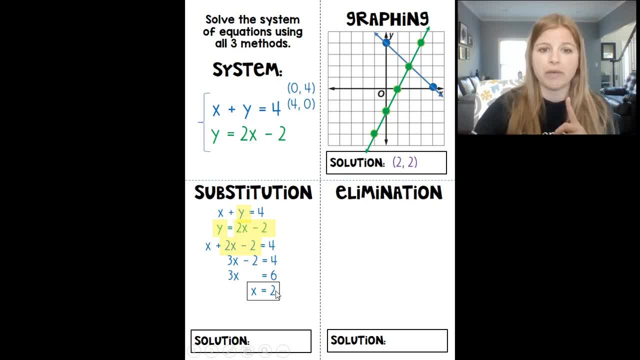 value. So if I have my x value, I still need to find my y value. So you can technically use either equation. I will always personally suggest that you use either equation, but if you need to solve for y, use the equation that's already y equals. So I'm going to use 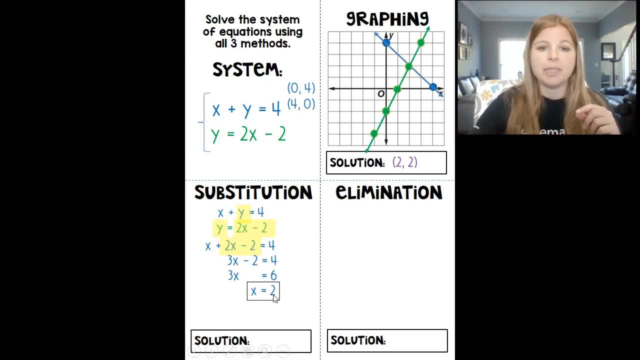 this equation: here y equals 2x minus 2, and I'm going to plug in or substitute this number 2 in for x. So instead of y equals 2x minus 2, it says y equals 2 times 2 minus 2.. 2 times. 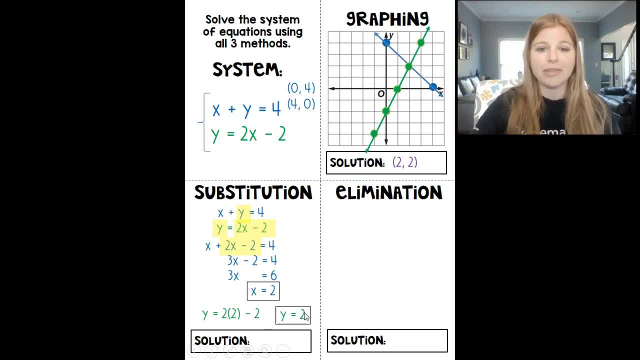 2 is 4.. 4 minus 2 is 2.. And that's my solution: 2, 2.. Last one elimination. So I'm going to take these two equations. I'm going to take these two equations and I'm going to. 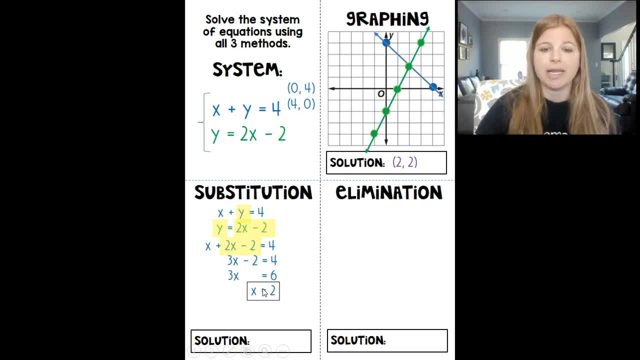 to get 3x equals 6,, divide both sides by 3, and x equals 2.. And that's wonderful. But let's remember the solution. when we graphed it was an ordered pair: It's an x and a y. 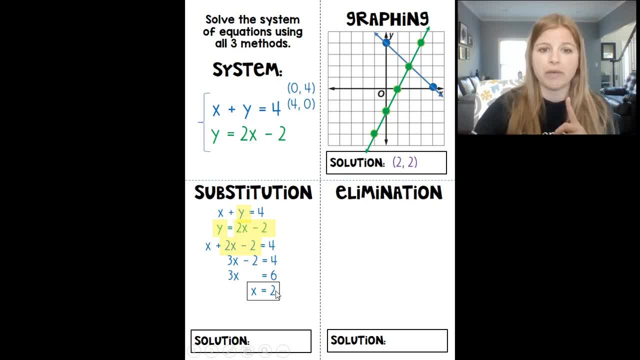 value. So if I have my x value, I still need to find my y value. So you can technically use either equation. I will always personally suggest that you use either equation, but if you need to solve for y, use the equation that's already y equals. So I'm going to use 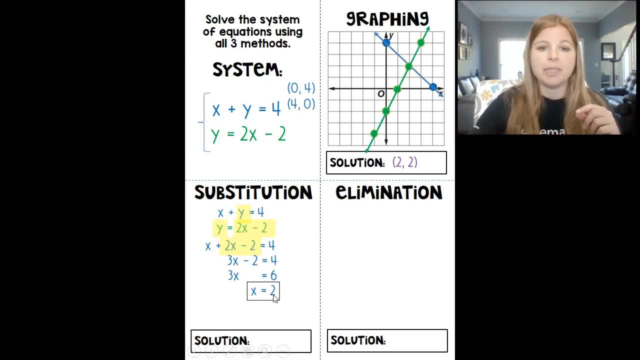 this equation: here y equals 2x minus 2, and I'm going to plug in or substitute this number 2 in for x. So instead of y equals 2x minus 2, it says y equals 2 times 2 minus 2.. 2 times. 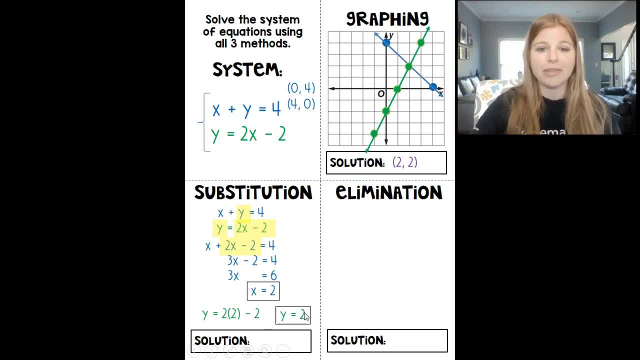 2 is 4.. 4 minus 2 is 2.. And that's my solution: 2, 2.. Last one elimination. So I'm going to take these two equations. I'm going to take these two equations and I'm going to. 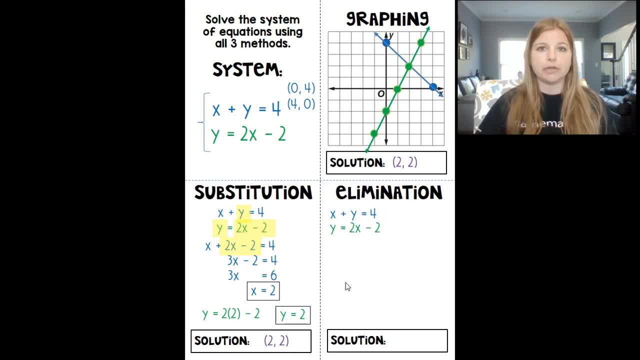 take these two equations Now. elimination works the nicest when both equations are in standard form. And the first equation is in standard form: x plus y equals 4.. So I don't need to do any rearranging for that. But our second equation, we know is in slope-intercept. 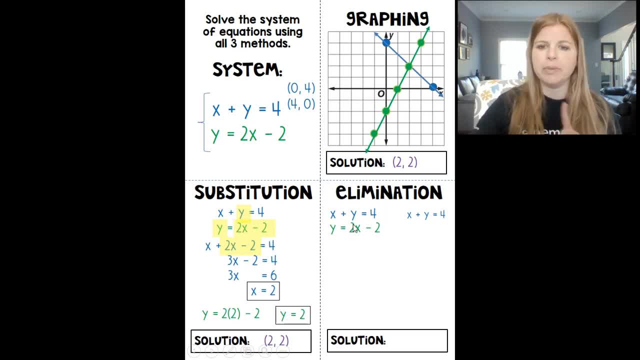 form, And in order to get that to be in standard form, I would need to move my 2x, my ax value, over to the left-hand side. So I'm going to go ahead and I'm going to subtract 2x on. 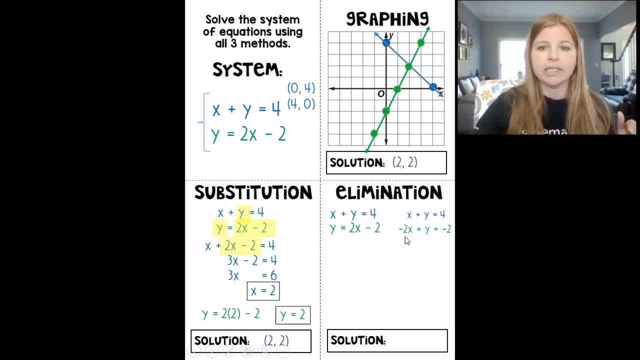 both sides, so that my equation now looks like this: Negative 2x plus y equals negative 2.. Now we learned for elimination that if I have opposite signs of the same variable, if I add them, they'll eliminate out. So if I was to add these two equations together, 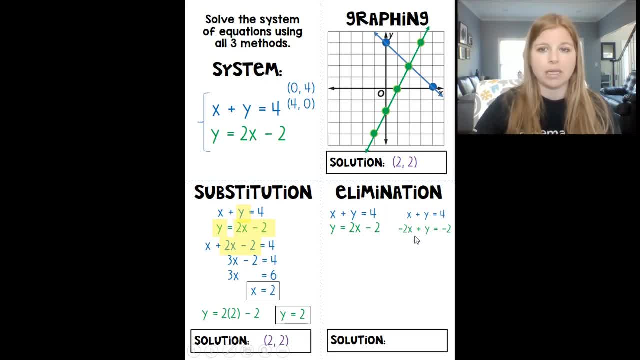 x plus negative 2x is a negative x That doesn't eliminate out. y plus y is 2y That doesn't eliminate out. So when addition doesn't work to eliminate, we use subtraction, Because if I do y minus y, my y's will eliminate out. 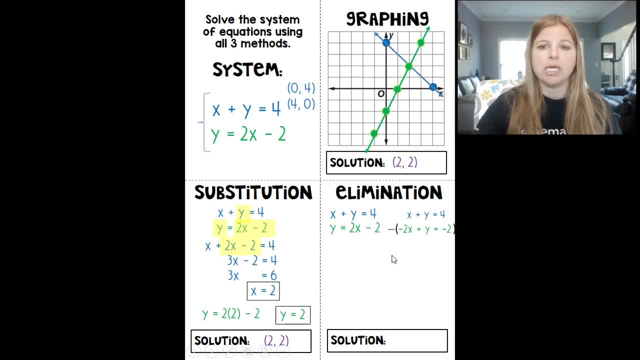 So what I need to do is I need to subtract the entire second equation. So I put a minus sign here, parentheses around the entire second equation, And we can go ahead and do the math. x minus a negative 2x really means x plus 2x, which is 3x. y minus y, that's. 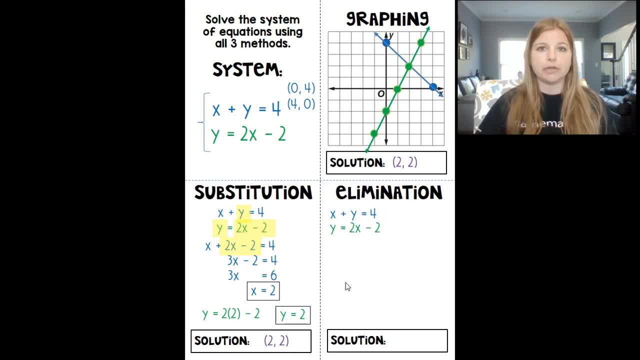 take these two equations Now. elimination works the nicest when both equations are in standard form. And the first equation is in standard form: x plus y equals 4.. So I don't need to do any rearranging for that. But our second equation, we know is in slope-intercept. 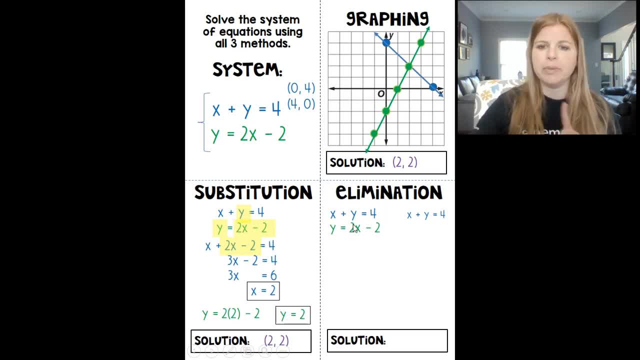 form, And in order to get that to be in standard form, I would need to move my 2x, my ax value, over to the left-hand side. So I'm going to go ahead and I'm going to subtract 2x on. 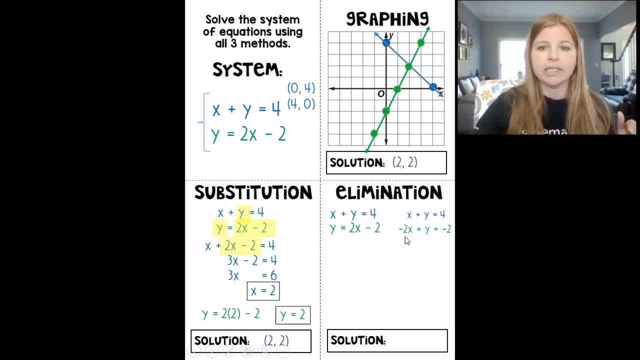 both sides, so that my equation now looks like this: Negative 2x plus y equals negative 2.. Now we learned for elimination that if I have opposite signs of the same variable, if I add them, they'll eliminate out. So if I was to add these two equations together, 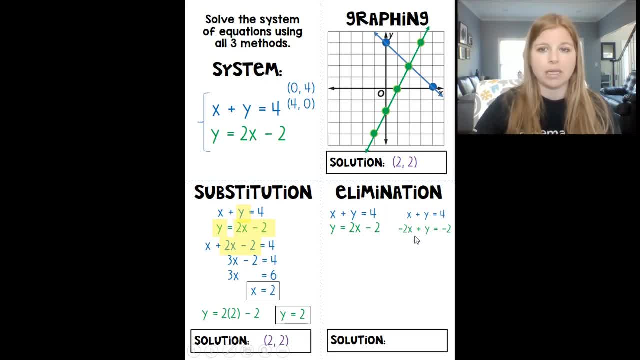 x plus negative 2x is a negative x That doesn't eliminate out. y plus y is 2y That doesn't eliminate out. So when addition doesn't work to eliminate, we use subtraction, Because if I do y minus y, my y's will eliminate out. 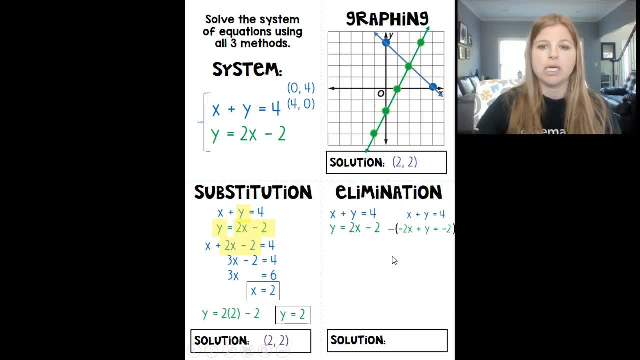 What we need to do is I need to subtract the entire second equation. So I put a minus sign here, parentheses around the entire second equation, And we can go ahead and do the math. x minus a negative 2x really means x plus 2x, which is 3x y minus y, that's. 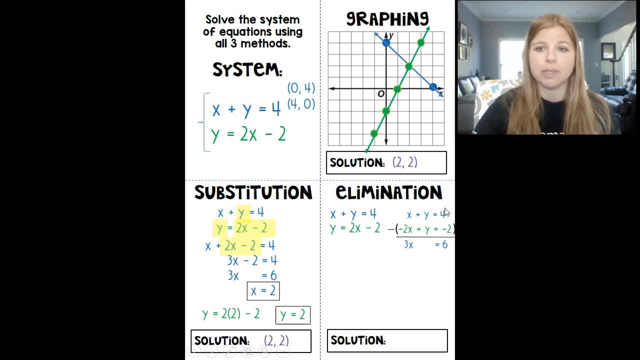 gone, And then 4 minus a negative 2 really means 4 plus 2, which is that 6.. And this should look very, very familiar, because we have 3x equals 6 here, which then leads me to x equaling two when I divide both sides by three and then just like: 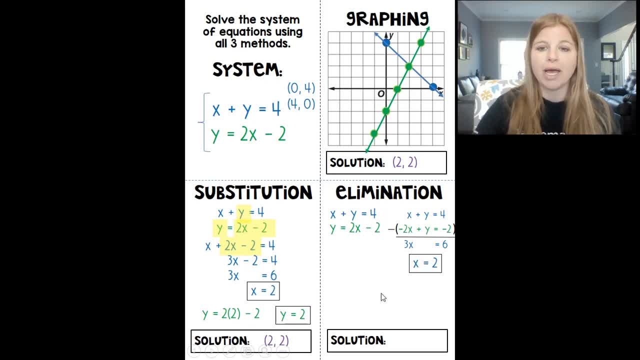 the same step here, guys. if I have x, that means I need my y. I'm going to go ahead and use the y equals equation. substitute that two in and I get two as well. if I had plugged in that two here for x, two plus y equals four, I'd also get that y was two. notice for each one of these different cases. 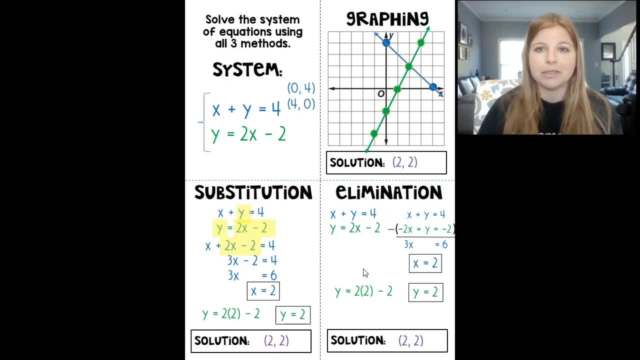 graphing. substitution or elimination, we all get the same solution. that's a really, really important skill to see and something to really make note of, because, let's say, I asked you to solve a system of equations and I said, hey, you must solve this by graphing, and you go ahead and you graph it.